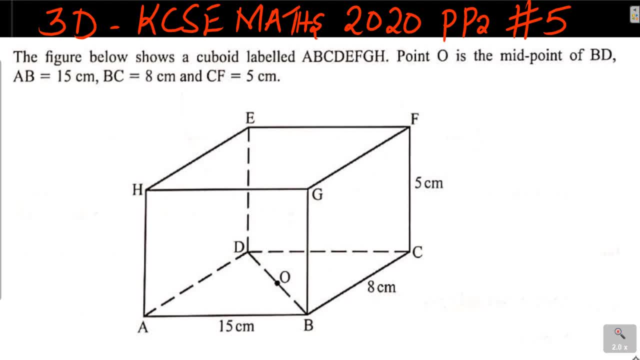 Hello viewers and welcome to the lesson three-dimensional geometry- KCC mathematics 2020, paper 2, question number 5.. The question reads: the figure below shows a cuboid labeled ABCDEFGH. Point O is the midpoint of BD, AB is equals to 15 centimeters, BC is equals to 8 centimeters, CF is equals. 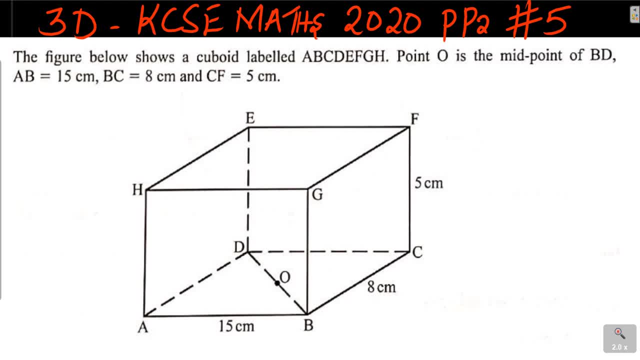 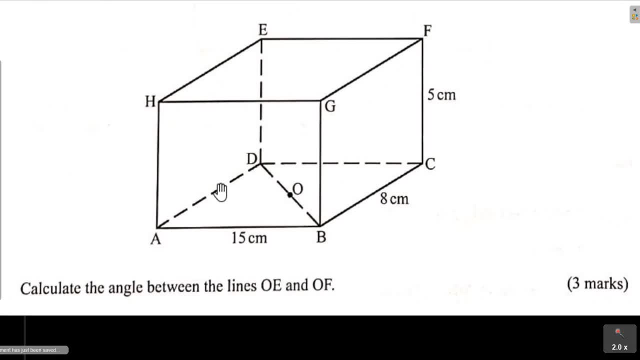 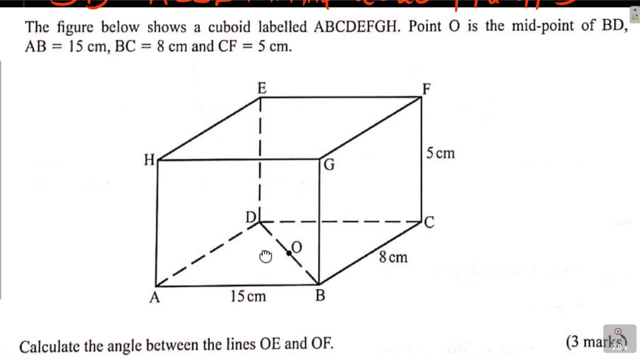 to 5 centimeters. So the diagram is here. You can see all the points. The question below it is: calculate the angle between lines OE and OF, The angle between OE and OF. So I will draw those lines, So I'll draw OF. So that is OF And OE. 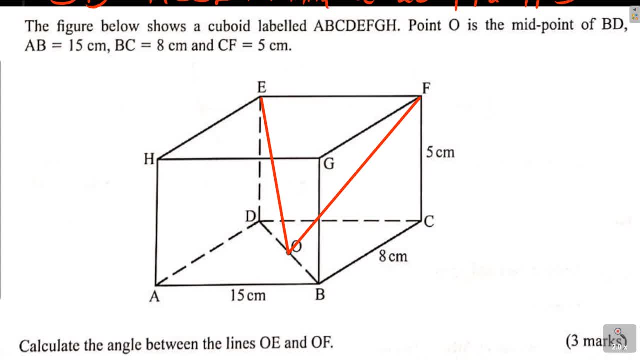 Now that we have drawn OE and OF, we are going to draw the angle between lines OE and OF. So I will draw those lines, So I'll draw OF. So that is OF And OE, Now that we have to see the required angle. And now those are the lines. So the angle required is this: 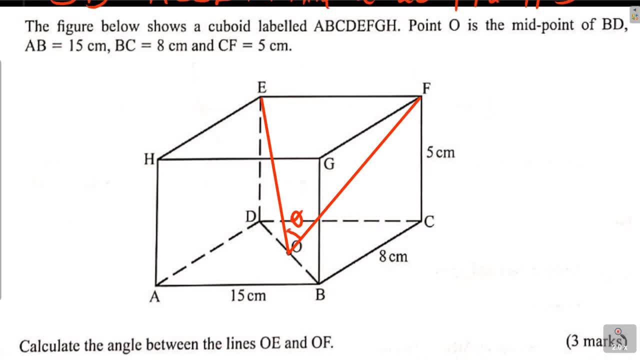 angle that is between. We can call that angle theta, The angle between those two lines. Having done that, there is something we need to get. We don't have the length OF and the length OE, So we need to calculate where it starts with OF. How do we get OF? To get OF. 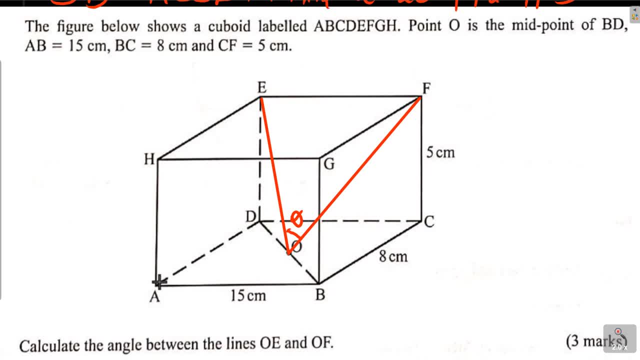 we will be required to get the length of this line. that is here AE or AC. This is line AC And then, when you get AC, it will be possible now to get OC, To be able to get OC. So now, having done that, let me- I think this one is a cuboid, or the base, All these. 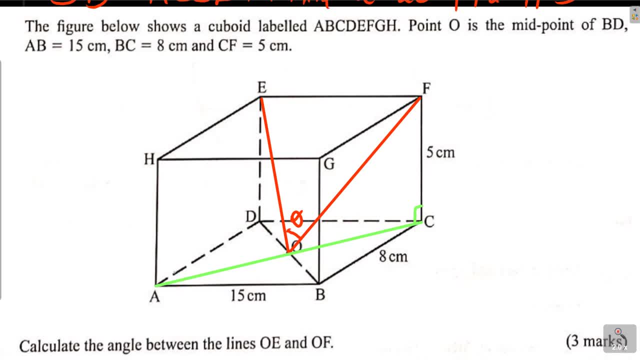 angles are 90 degrees. these are corners. here, these angles are 90, this one is 90, this one is 90 as well, and this one is 90.. Now, using triangle ABC. using triangle ABC, we can get AC. so AC will be given by using Pythagoras theorem. this will be 15 squared plus 8 squared. 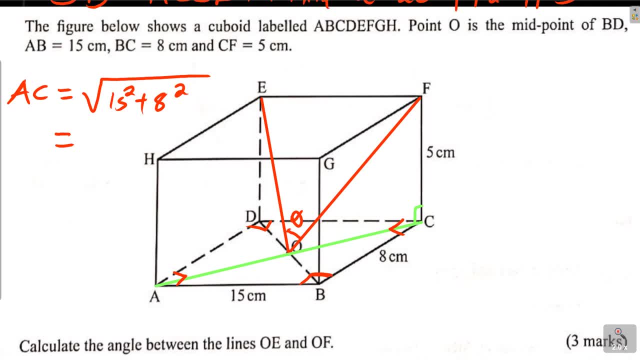 and this one will give 15. squared is 225 plus 64. this will give the square root of 289, and when you get the square root you get 17. so AC is 17.. O is the median point of that line. Therefore, OC will be half of that and this will give 8.5 cm. So this 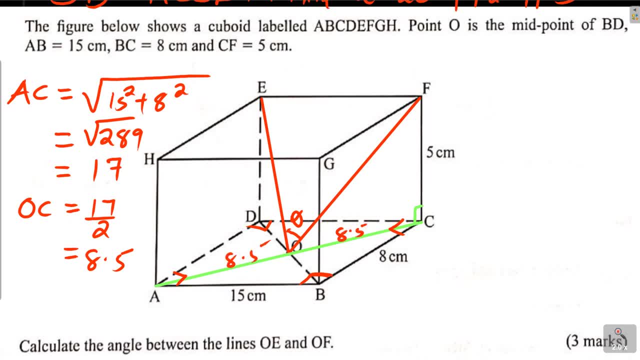 one is 8.5 and this one is 8.5.. Now look at this triangle. Now OFC, OFC will make it possible to get OF. So, considering that triangle, OCF will be able to get OF, So OF now will be. 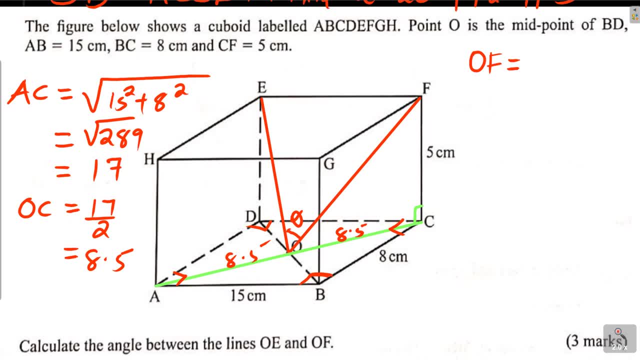 given by OF, that is the hypotenuse paradigm theory. we shall use 5 squared plus, since that is the hypotenuse 8.5 squared. 5 squared plus 8.5 squared, that will give 99.25. and when you get the square root of these square root of 99.25, 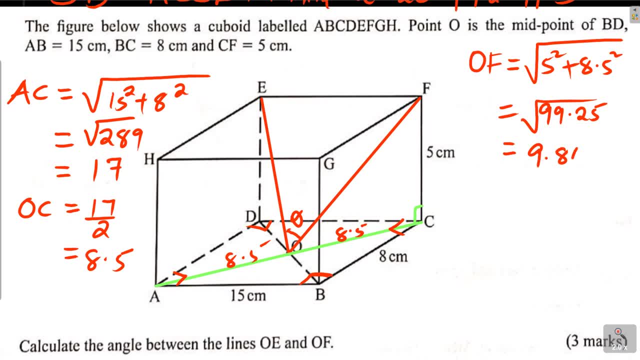 which will give 9.862 centimeters. so this one is 9.862. now we have obtained of, now let us get oe. now to get oe, you'll notice that we're required to get um. consider this triangle: oed, oed. already we have de. de is five and um db. db is what you need to get. and then when you get half of that, 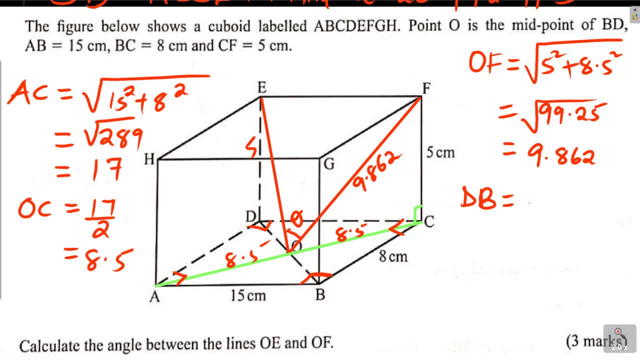 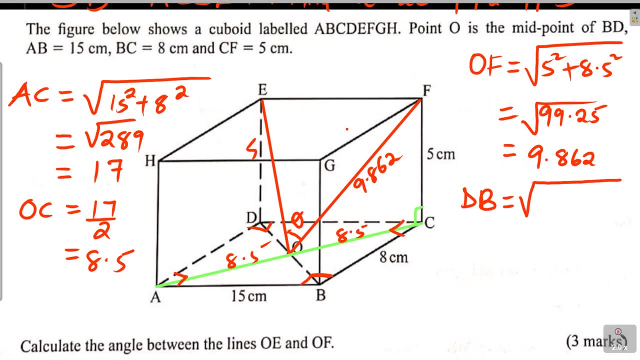 and you notice that db will be obtained the same way we obtained ac. so db. consider triangle dab, dab. you notice that db is the hypotenuse, so db will be given by considering triangle d. this is a dba. it will be so. we have ad. ad is eight. 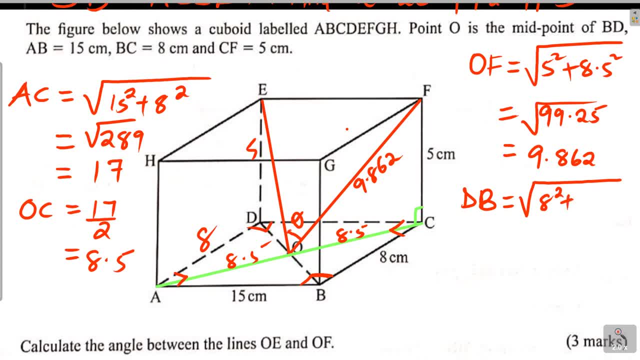 so it will be eight squared plus 15 square. you notice that it will be the same way. we obtained ac, so db, the asymptotic, is the dipd in the right side, and because db is equal to seven, we have to calculate it d inside d, so we'll 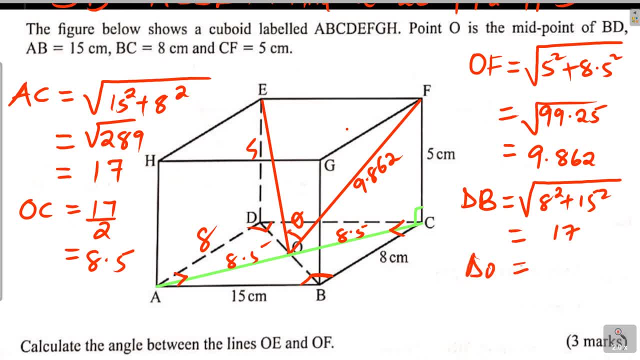 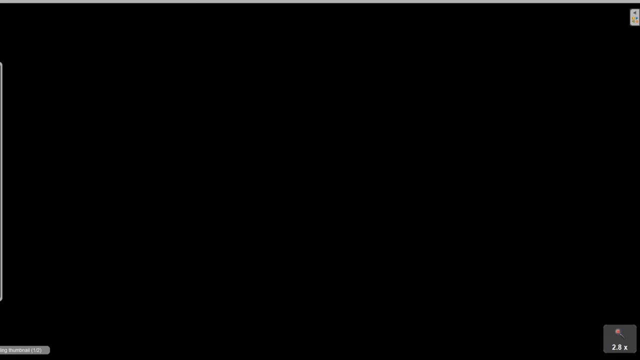 have uabalind for db and this is going to be ourized to d and then this will dis i, for this will be your d, this will be one makers straight line. so again, db a. so you come here and you'll lucky. or from the square root here, so we came by the othericAhd and we see thisdb again. 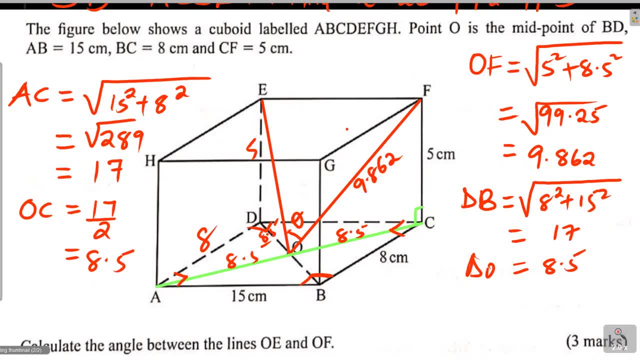 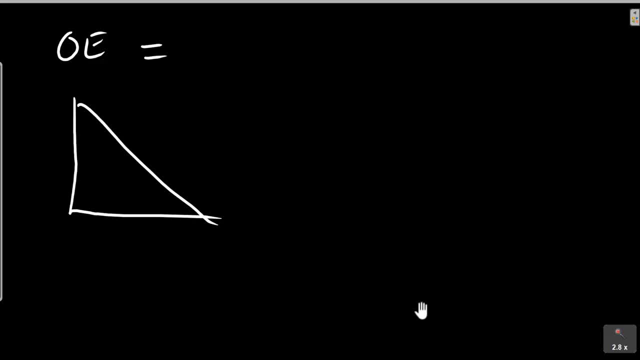 and we get here. since we had calculated this db will be 17 and therefore do do will be one half of. we have calculated these will be 17 and therefore do, do will be half of. O E. we shall consider triangle: E, D O, E, D O. 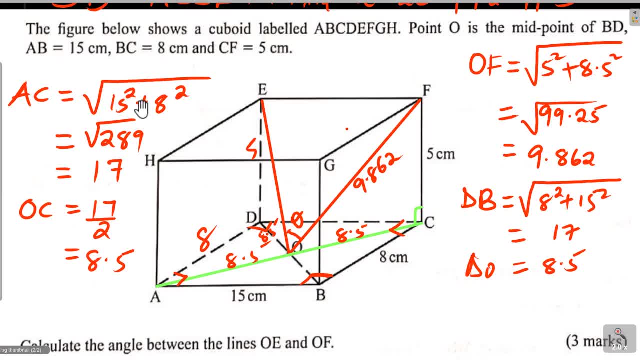 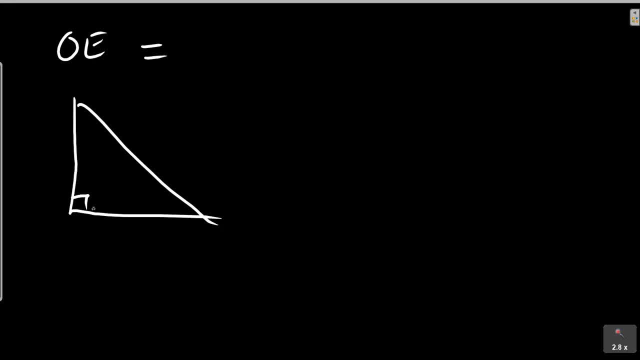 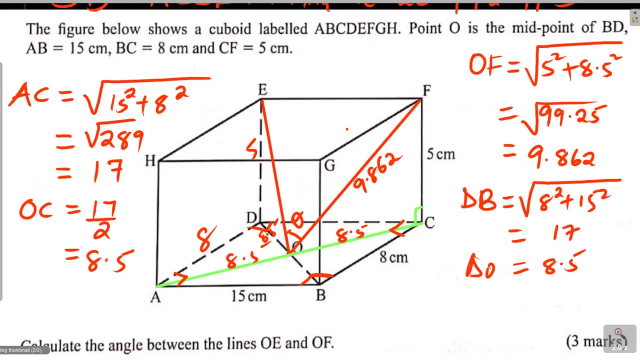 So to get O, E, we shall consider triangle: D, O, E, D O E. I'm just sketching it here. So we have 90 degrees at D, then this one is O and E is here. Let me just sketch: So D, E is 5 and D? O is 8.5.. 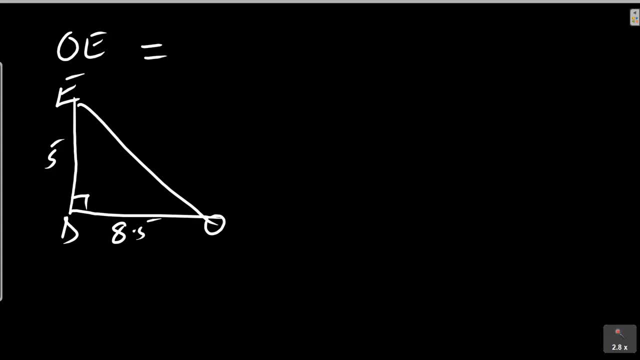 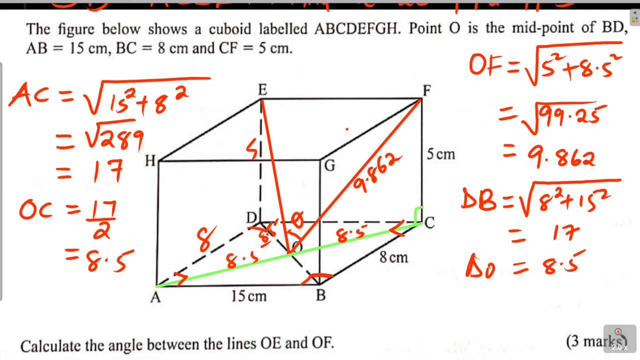 You've got that here: D O 8.5.. Now O E. using Pythagoras theorem, O E will be given by the square root of 5 squared plus 8.5 squared, And you notice that this is the same thing that we did to get O F. 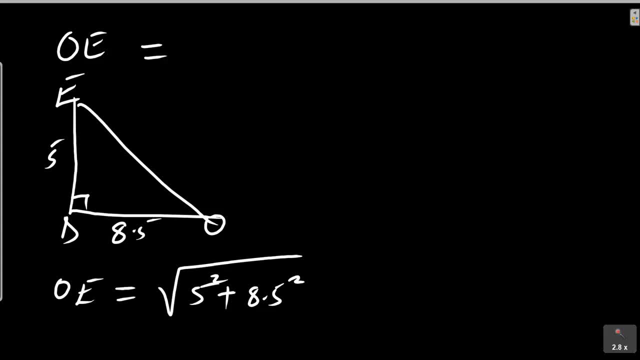 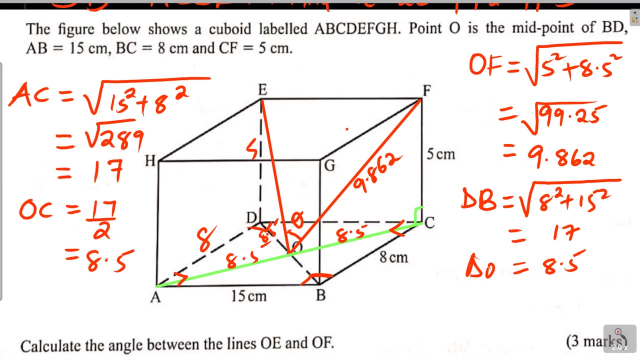 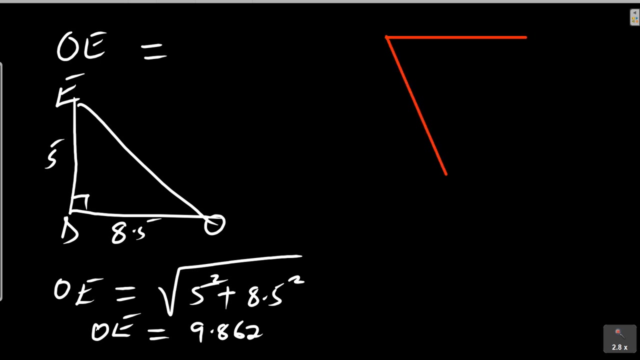 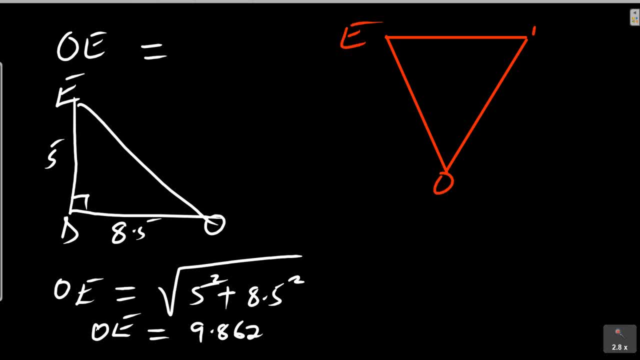 it here. So O, This is E and this one is F. So we have O E- O E is 9.862 and O F. we got O F again as the same thing, 9.862.. Now the angle that you require is the hole of this angle that is at the center between 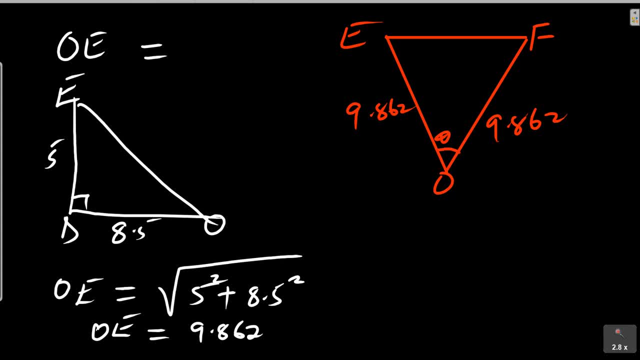 O E and O F. Now to do that. if this one is, if we do that, This one is 9.862.. This one is 9.862.. This one is 9.862.. If I draw that line there,